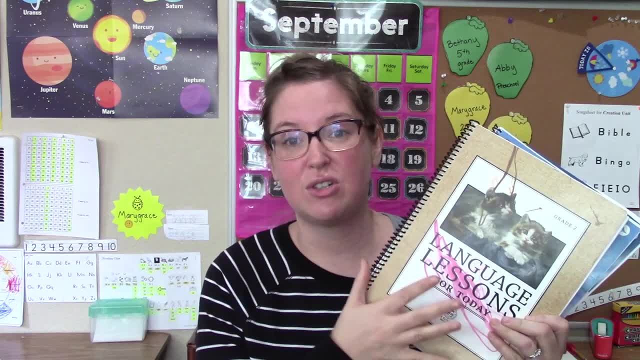 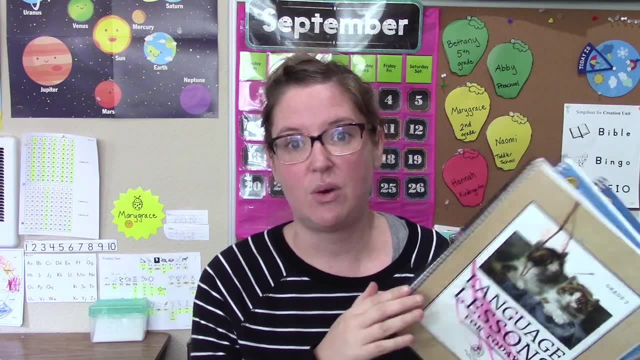 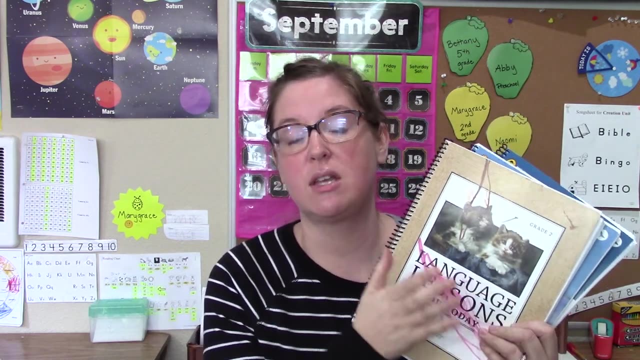 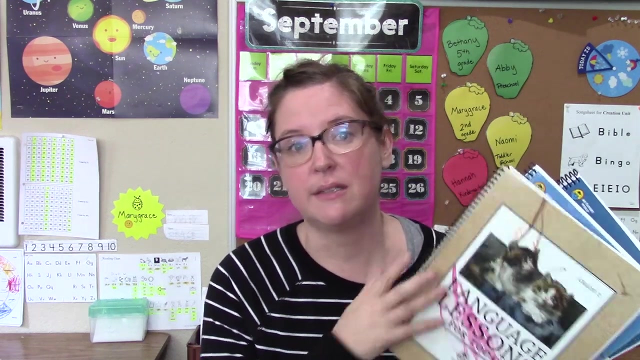 So I'm going to swing my camera around to show you kind of a closer look of what's in the books and then what can be explained. So it's really nice because they explain what the child will be learning each year and what's expected of you as a teacher. And I'll kind of tell you how I've modified things, if I've needed to, from child to child. 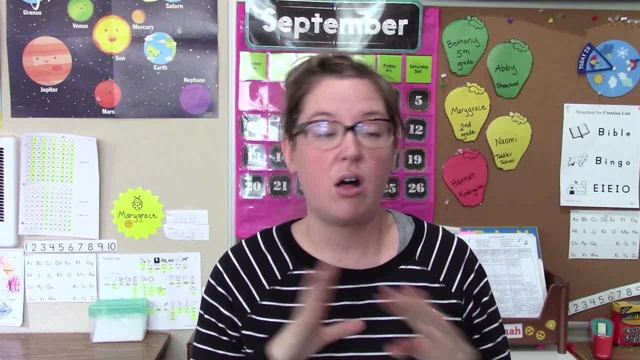 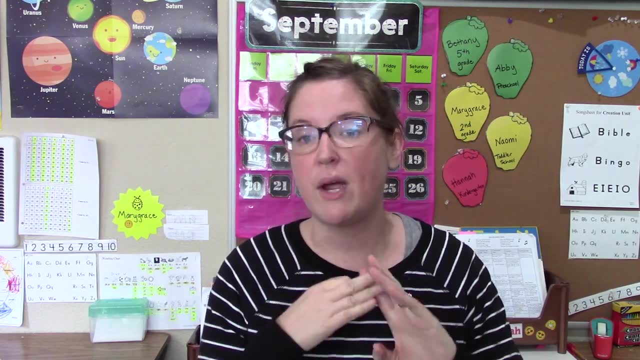 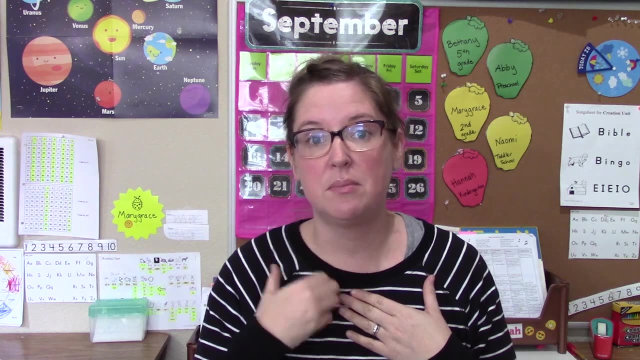 I've also been asked to share all of our, the whole language arts program from My Father's World, So that's including spelling, writing, grammar, handwriting, and I'm not going to share it all today because, first of all, we haven't used it all. um, we've used up to grade five everything that they. 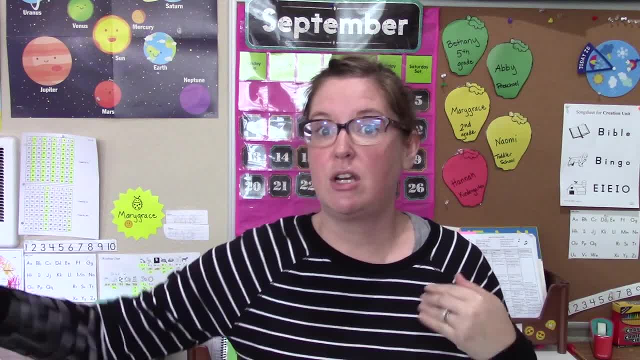 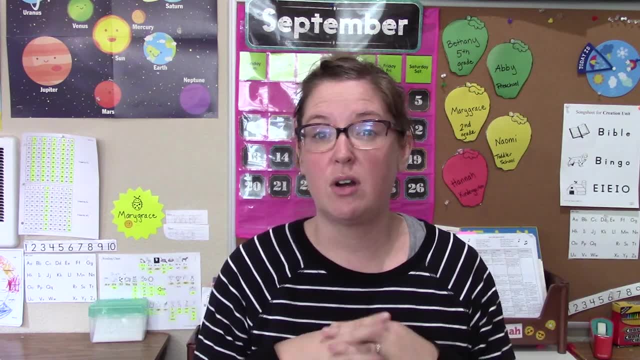 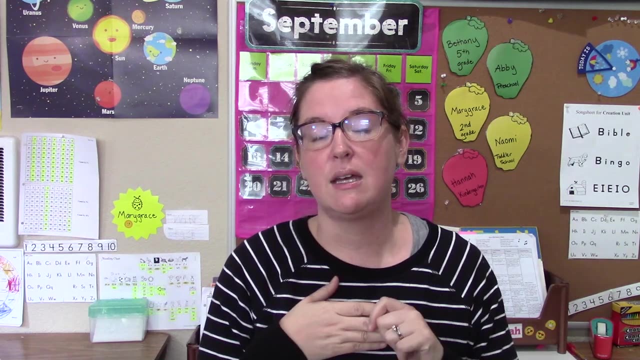 have um recommended, but it goes on and on through the junior high years and we're not to that, and so maybe i'll share what i have so far, if, if you guys are interested in something like that- that- what i have taught for their language arts program and um, but i'll be able to teach way more in years to. 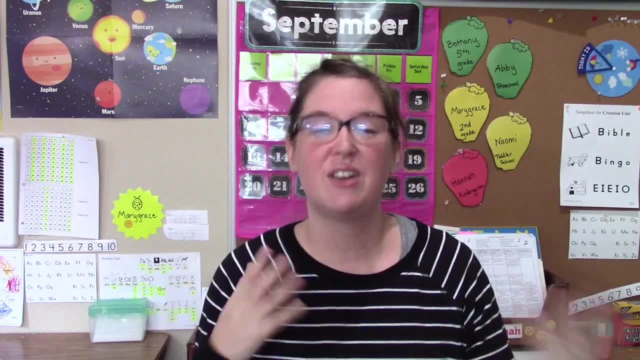 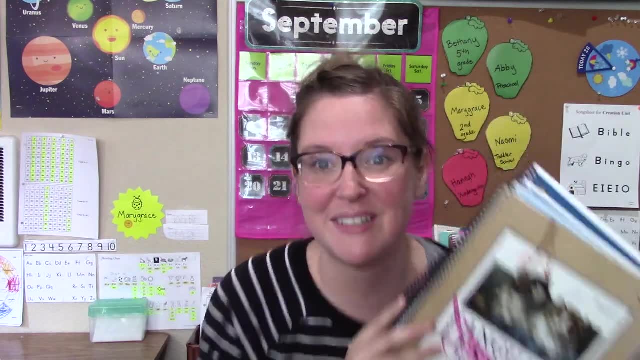 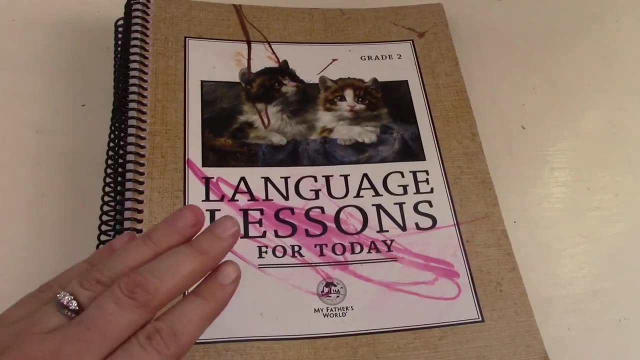 come, i shouldn't say teach, share with you more years to come after i've taught more, lord willing. so all right time to turn the camera around, okay. so now we're to the desk and i can share with you all the great books. so the newer language lessons for today, uh, for grade two has lions on front. 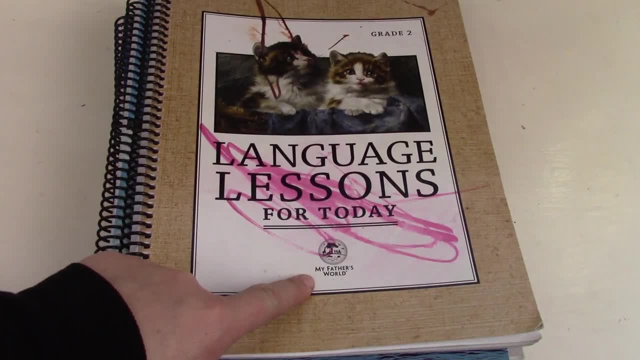 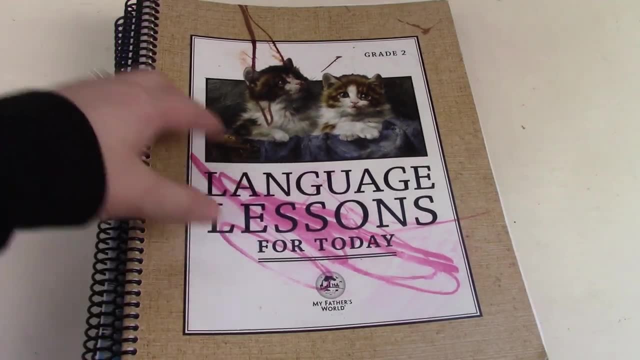 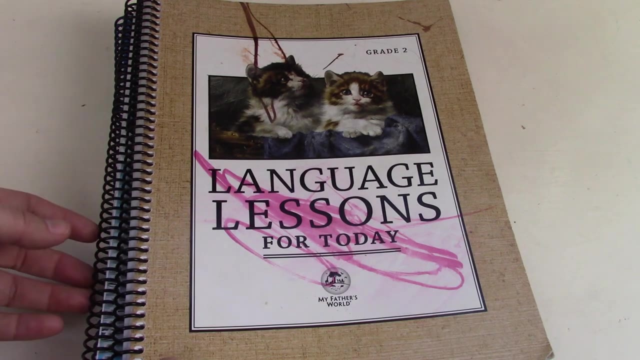 this is the older version, um, still from my father's world, and i'm not sure. i don't think that there's any changes except for the covers, but i will share with you what's in this one and then, if you get the new grade two- and it might be different, just be aware, okay, so we'll start with. 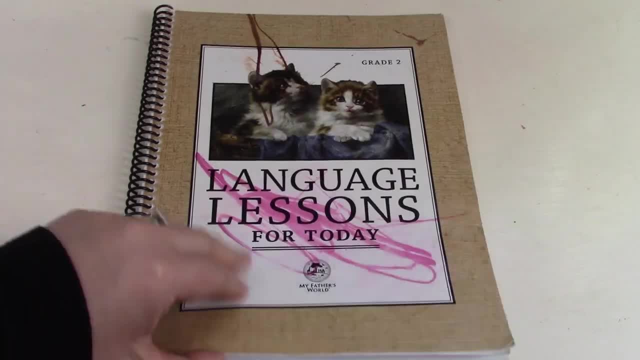 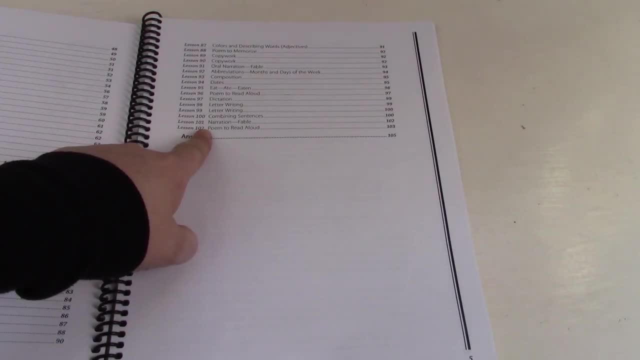 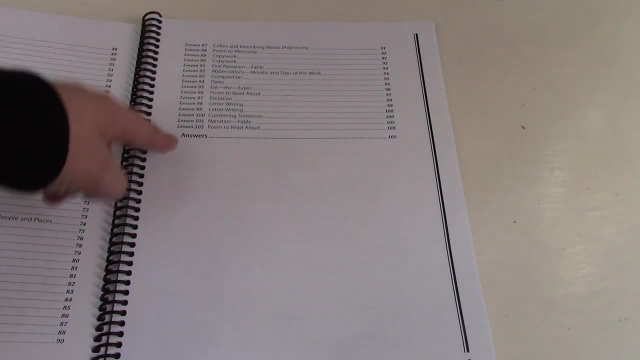 grade two, and then we'll go through each of the grades that i have so far. okay, so in grade two you have a total of 102 lessons, and it's really nice because in your teacher's manual, for whatever grade you're doing, it tells you you pretty much do only three lessons and then you have a total of. 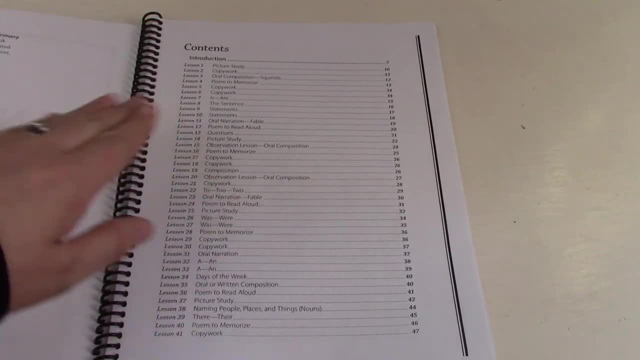 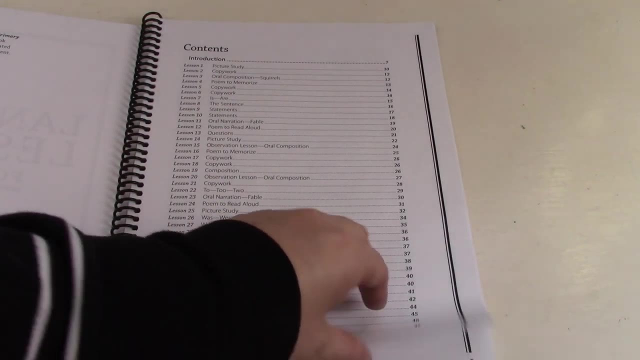 lessons a week, so that's really nice for the kids that they get like a day or two off from it. my kids don't typically mind the amount of work that they have in this, but sometimes if you don't have a big writer or kids that are super interested in language arts, 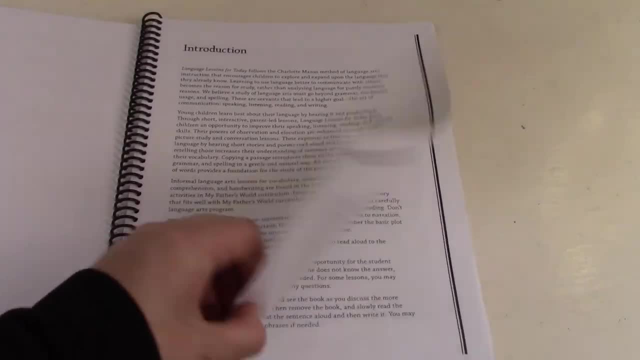 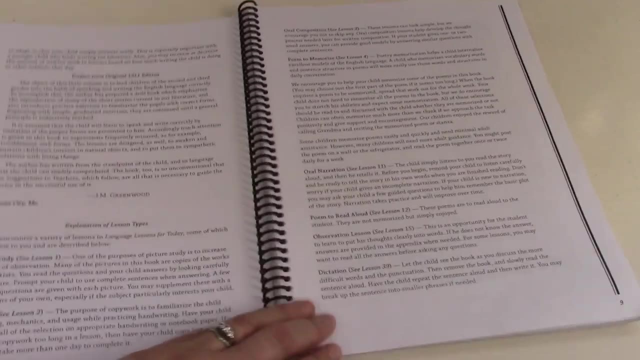 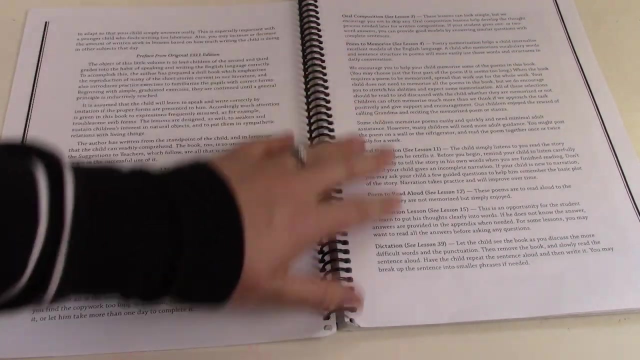 sometimes it can be a bit tedious for them. so there's a whole introduction on how it's set up and i like this part the best because it gives an explanation of the lesson types. so you'll do through this and it will tell you like which lessons to go to. 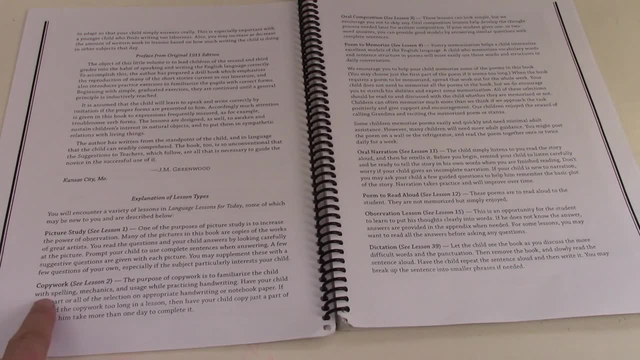 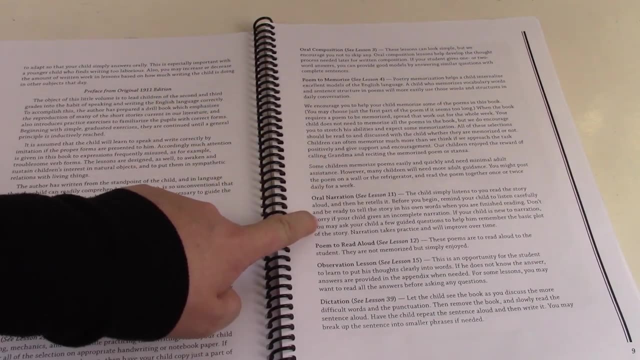 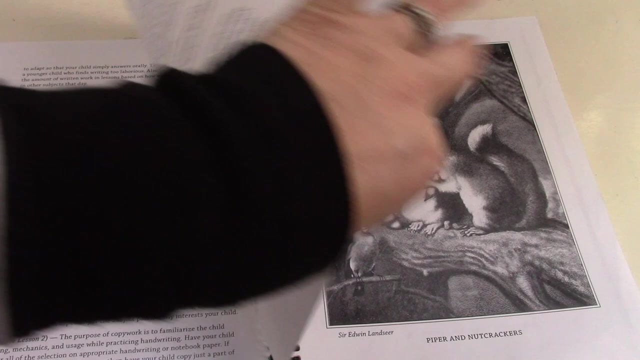 for an example of them. so we have picture studies, copy work, oral composition, poem to poems to memorize, oral narration, poems to read loud, observation, lesson dictation, and that's it. so that is the preface of what they'll be learning through the year and the different kinds of lessons. 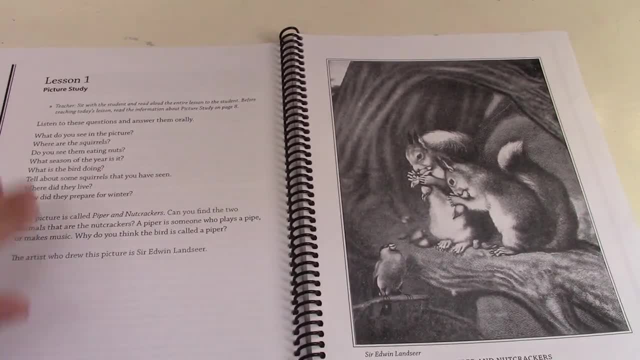 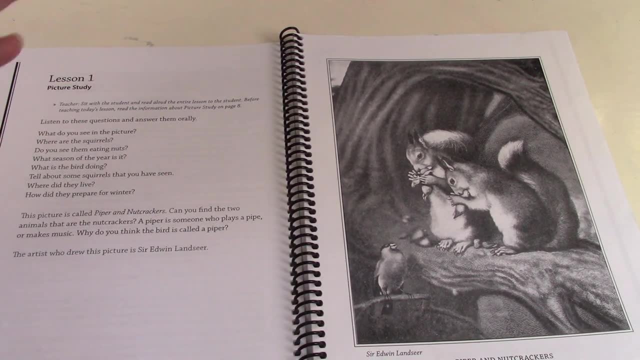 and it's really nice, because it's just really nice to be able to go through all the different lessons, because it's just laid out super simply. um, you have lesson one. they do a picture study, so here will be the picture that they'll study and then you'll have questions and it typically takes 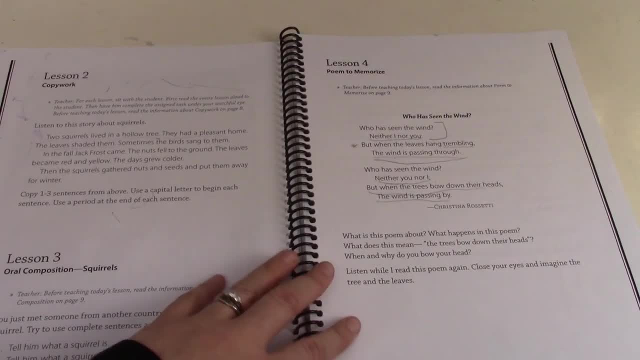 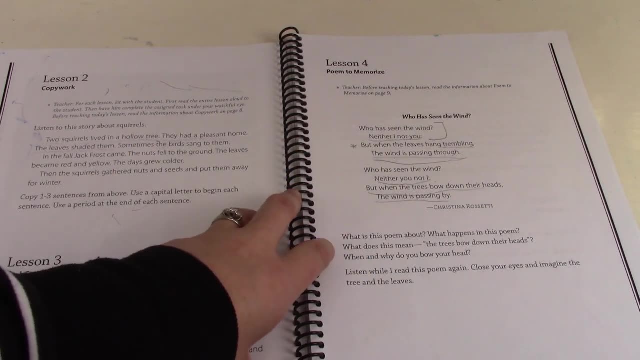 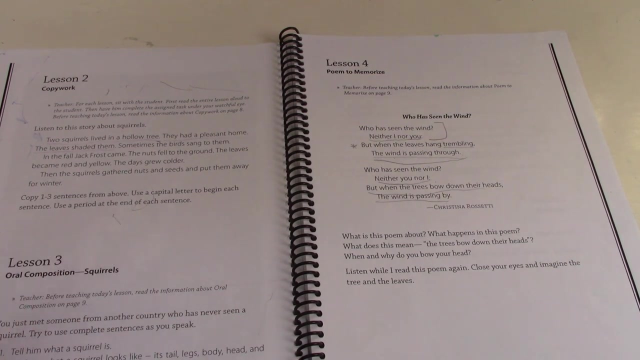 no more than 15 minutes. i have found sometimes way less than that copy work. these are poems to memorize. now for my grade 2. i don't typically always make them memorize or do all the copy work. i'll typically let them do less, depending on the student i have. if i have one, that doesn't mind. 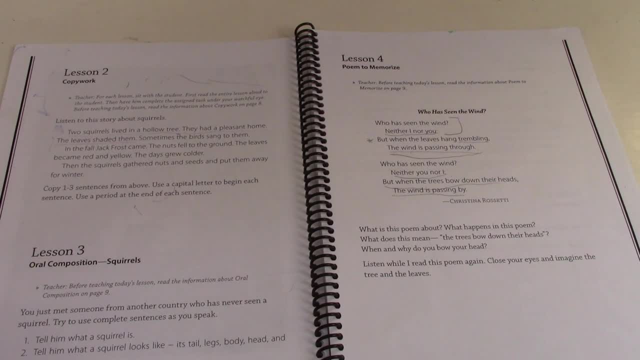 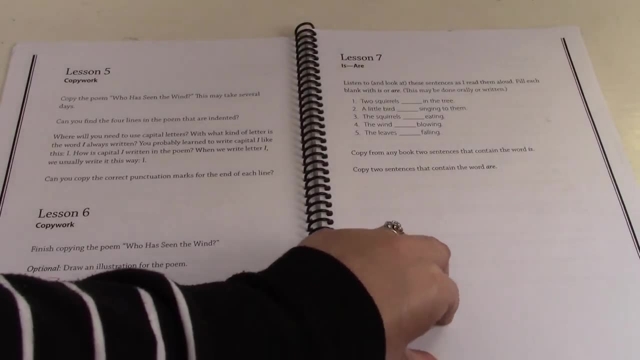 I'll do more, but I've had one that is not so much into the writing, so I try and keep it still fun, I should say. so there's just a lot. I'm not going to show you every page, but you know here's another poem to read aloud. I really 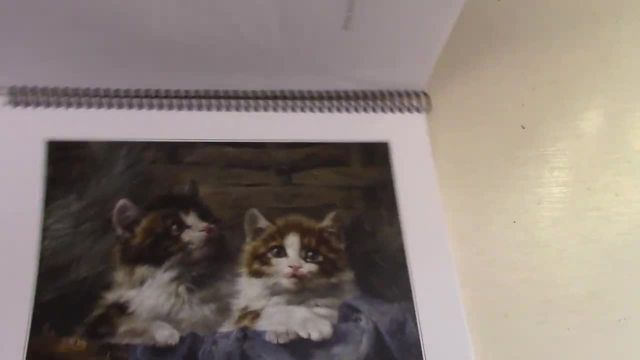 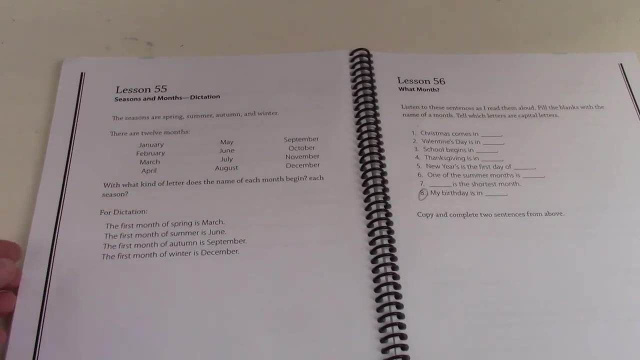 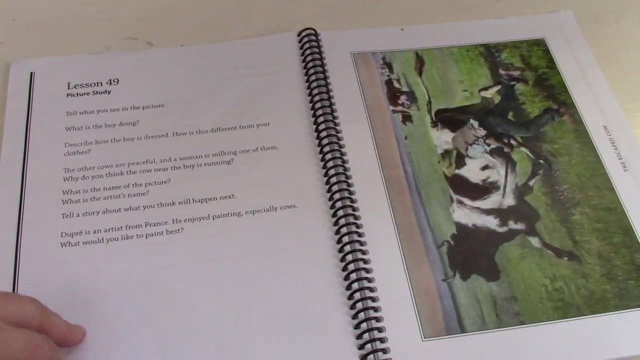 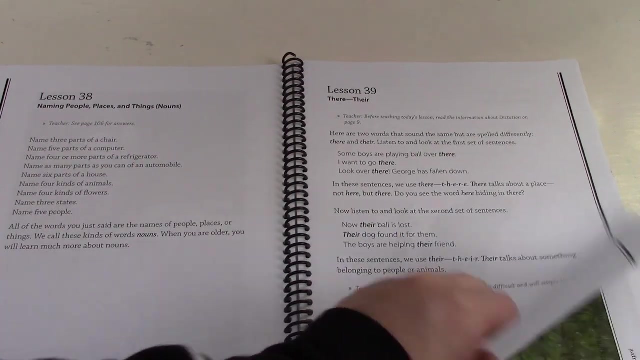 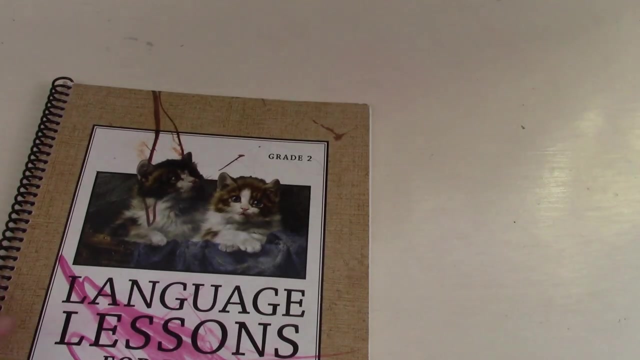 always, I always love the picture studies. those are always our favorites. but they'll do things like learning about the seasons and the months. another picture study: they'll learn the differences between there, there naming people, learning about nouns. so it's just a really gentle way to learn grammar in language arts and I just really, really 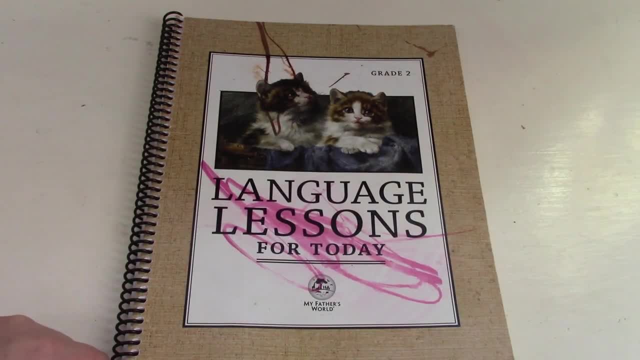 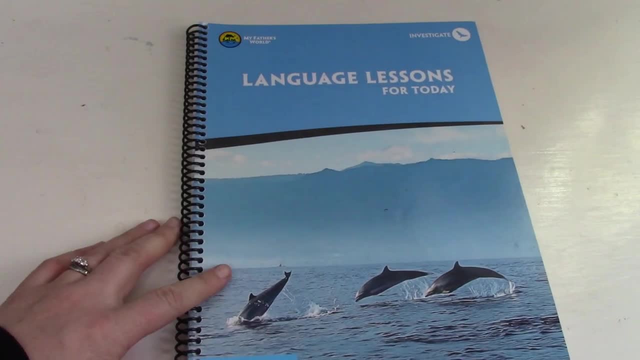 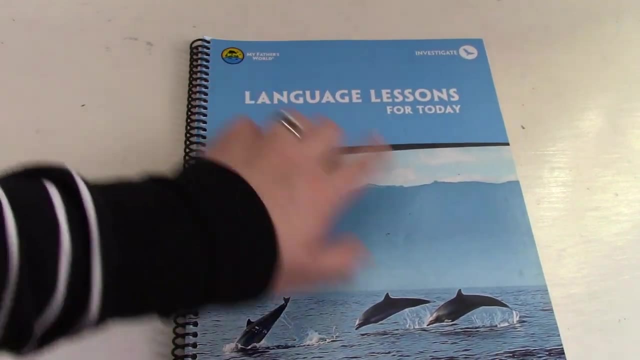 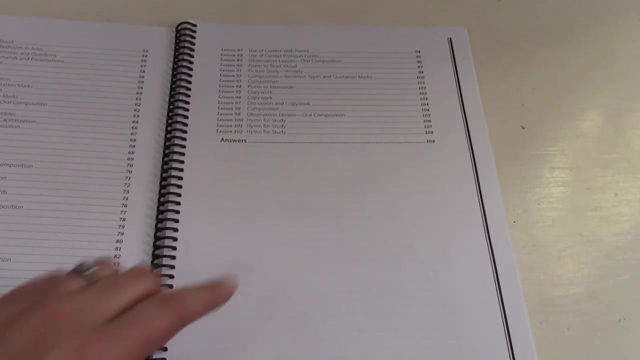 love. I really love this language lessons. I can't say more about how great it is. so that was great too. now each level will build upon itself, each grade, I should say. so here's language lessons for today, level grade three, again from my father's world, and again here's your content and a hundred and two lessons. so. 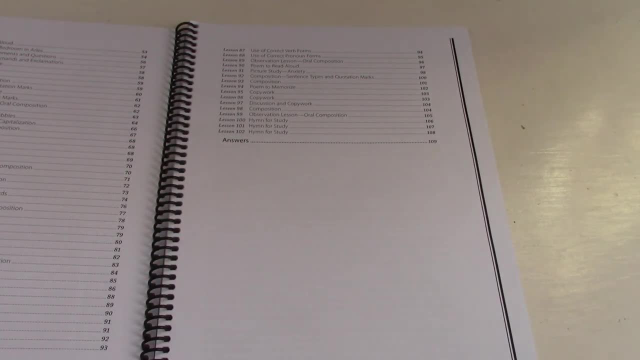 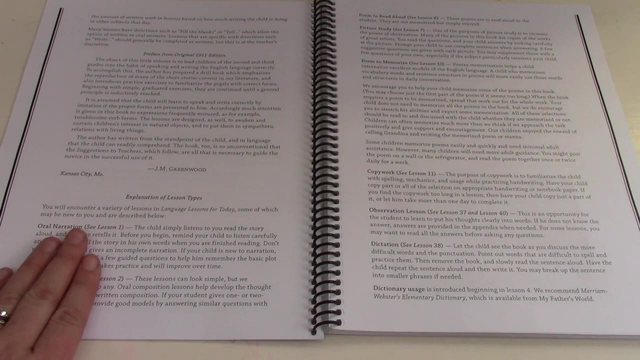 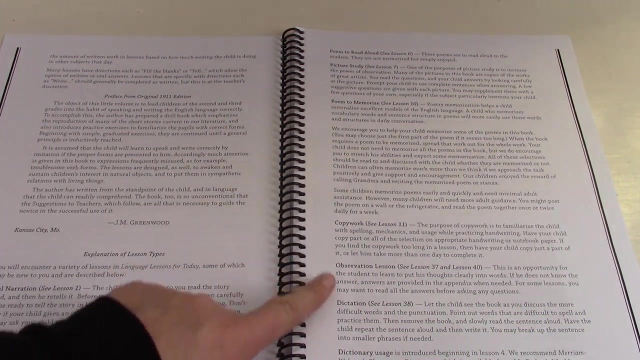 I believe it's the same amount, yep a hundred and two lessons. so again you have your introduction on how to do things and then an explanation of the lesson type. so again you have oral narration, oral composition, poem to read aloud, picture study poem to memorize, copy, work, observation lesson. 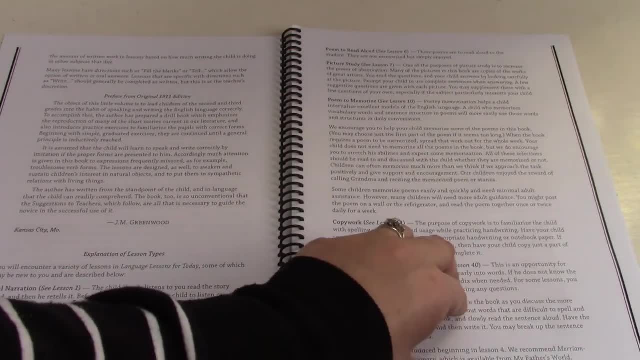 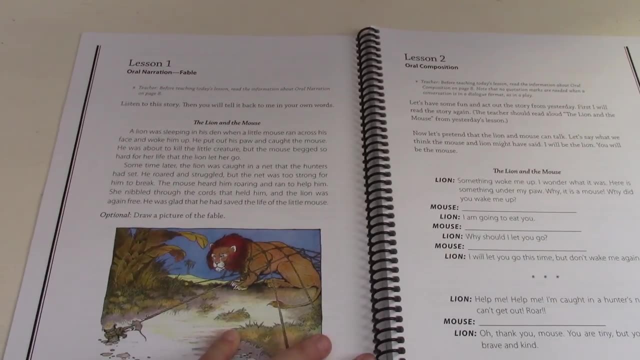 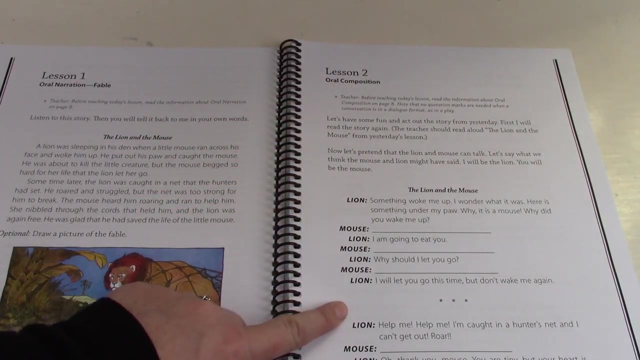 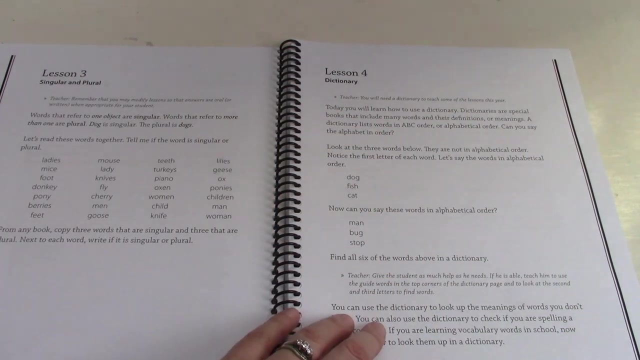 dictation, dictionary usage. so this year you start dictionary and then we go right into it. so here's an oral, oral narration of a fable and at the end they can draw a picture. then we come over here and there's an oral composition and it ties into this line in the mouse story, and then we have dictionary use. 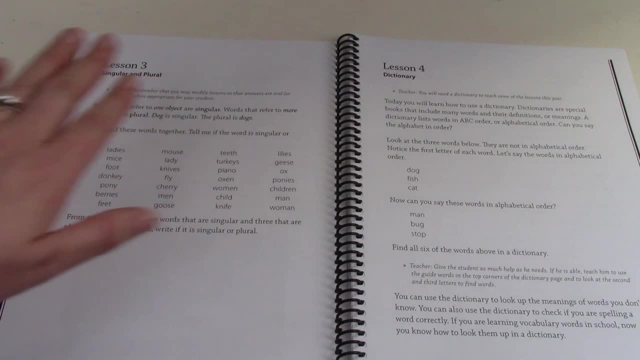 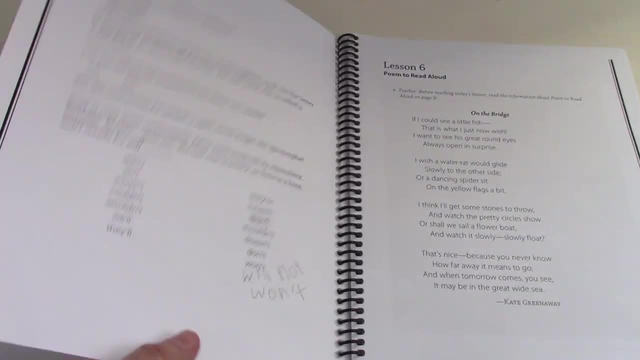 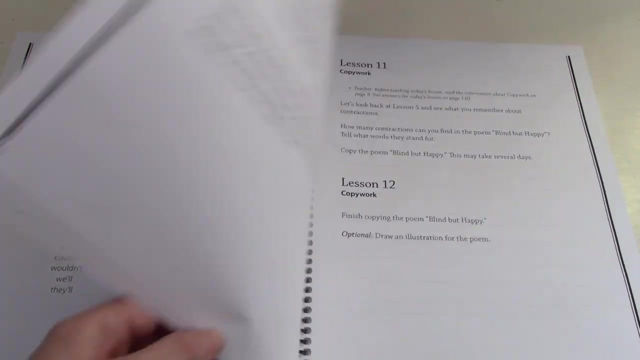 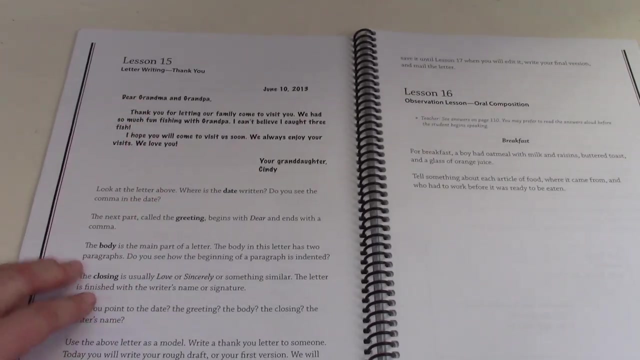 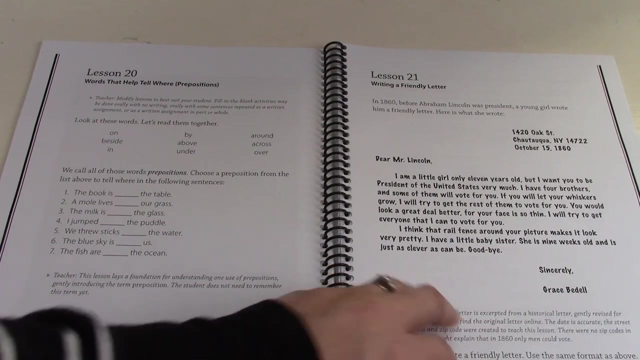 and learning about singular and plural, and it's all just very late, laid out very easily and very simply to teach. again, here's a poem, obviously added a little bit in here. more poems, copy work, how to write a letter. that's always great to teach because this kind of becoming a lost art, more letter writing learning. 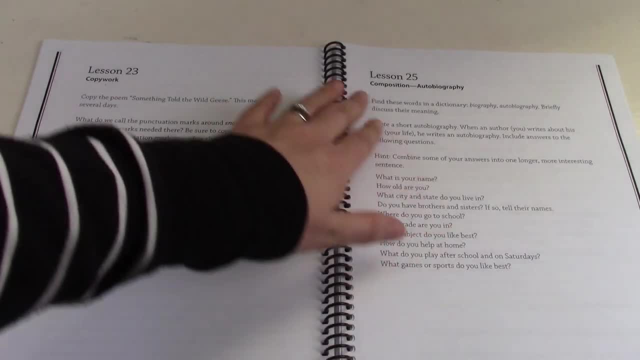 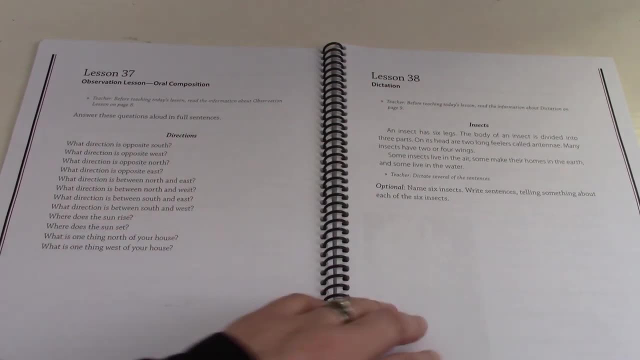 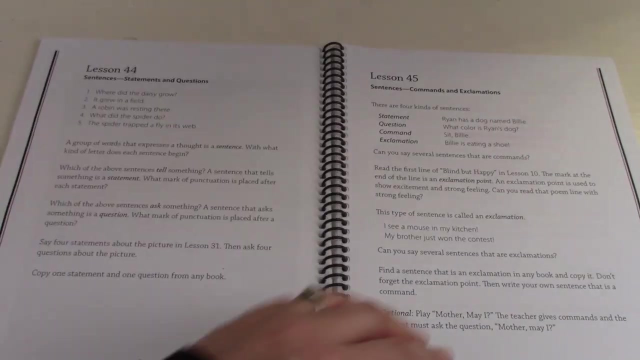 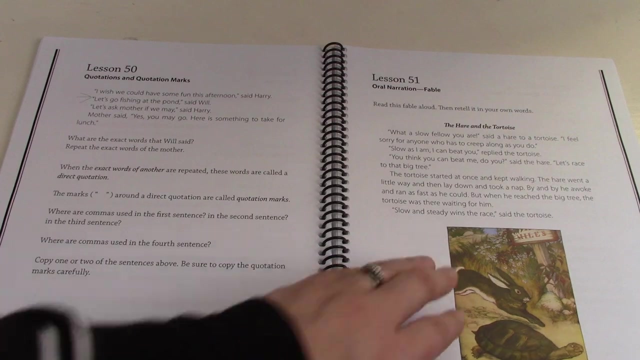 about prepositions, composition for an autobiography, dictation, observation lessons with oral constitution, more poems, learning about synonyms, and you're really just building a little bit from the second grade to the third grade. And that's what I found, Jake. It's just a little bit more and then a little bit more. 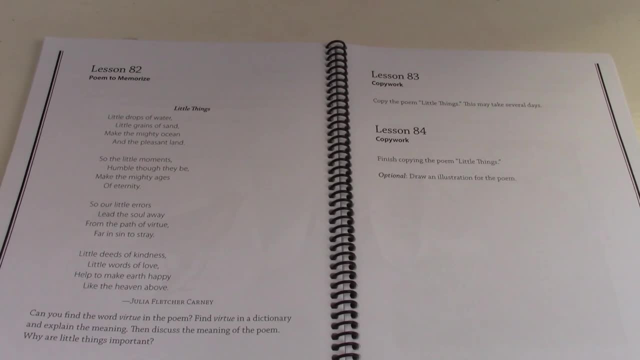 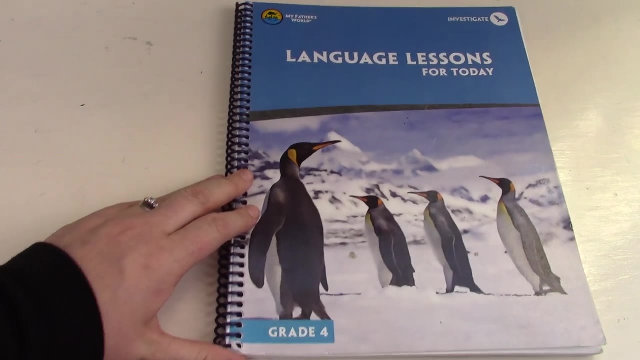 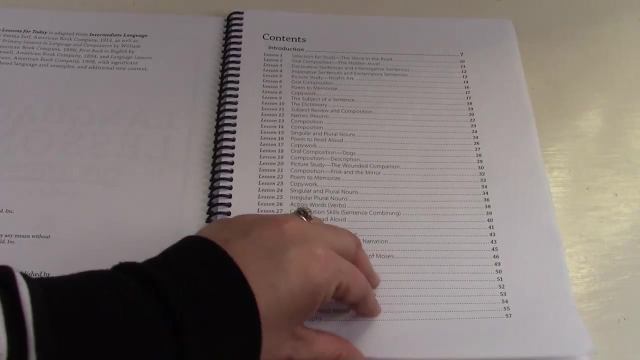 And so here's some vocabulary, and there you go, Some more poems and copy work. So that was grade three. Okay, moving on to grade four, Language lessons. for today. again, We're just building a little bit. more. Okay, so again, our introduction and our contents. 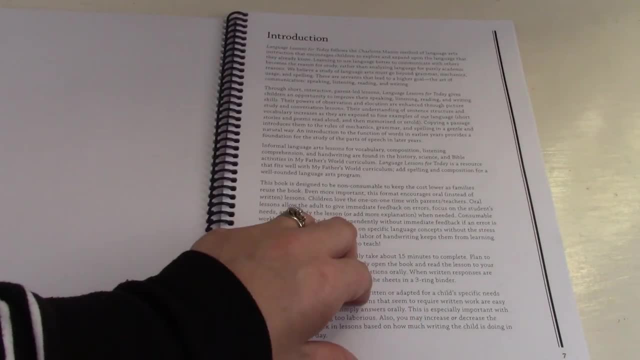 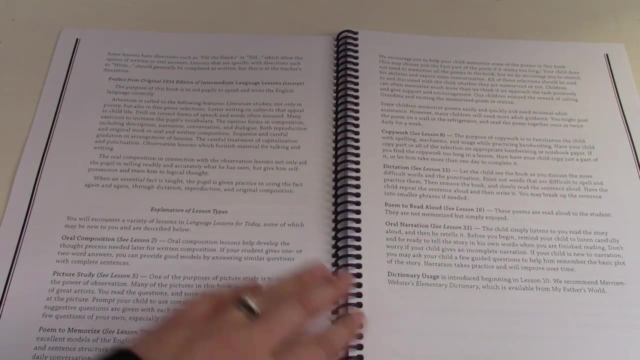 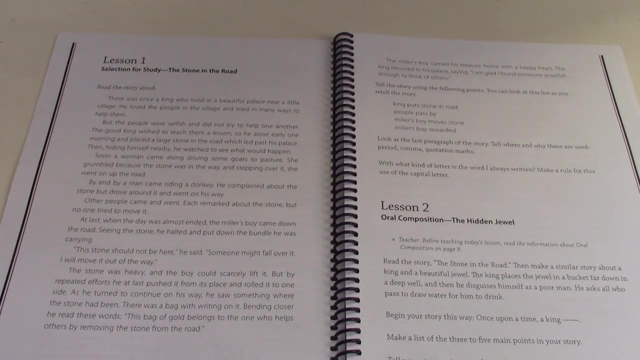 Oh, I say content. So again, 102 lessons, your introduction, And again it's all the same here that they're learning poems to memorize, copy work, dictation, dictionary usage. So again right to lesson one: selection for study. 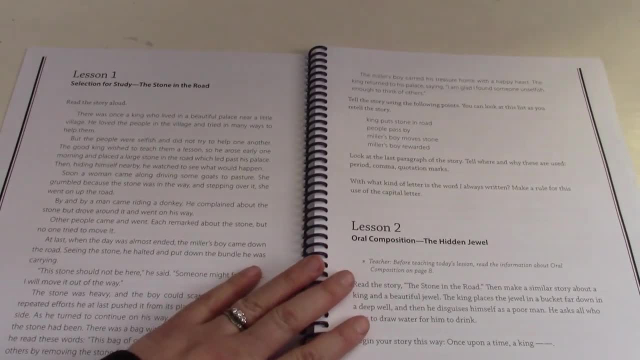 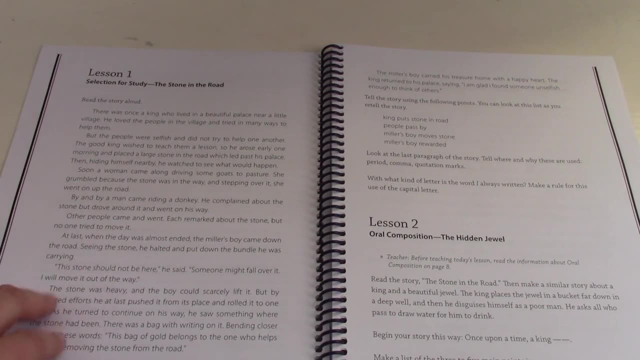 So you read the story aloud to them and then they look at the paragraphs and they're learning what kind of letters like, how a paragraph, how a paragraph is started with the capital letter. There's periods and commas and quotation marks, Making a rule for the capital letters. 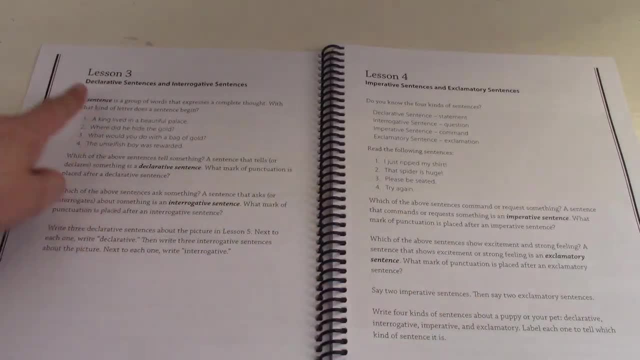 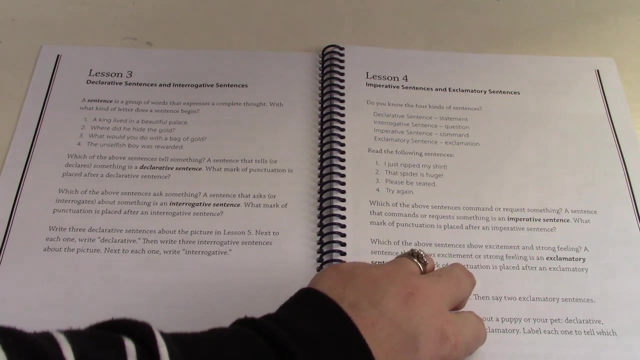 and there's an oral composition. They're learning then about declarative sentences and interrogative sentences and imperative sentences and exclamatory sentences. lots of sentences, And then picture studies- my favorite, Aren't they pretty? I love this one. 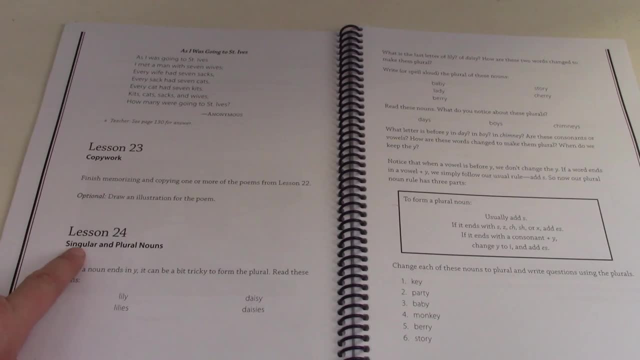 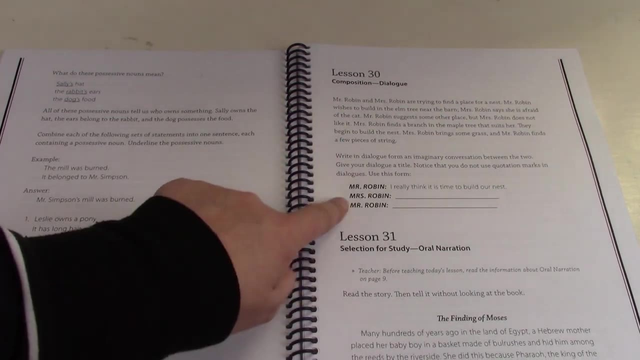 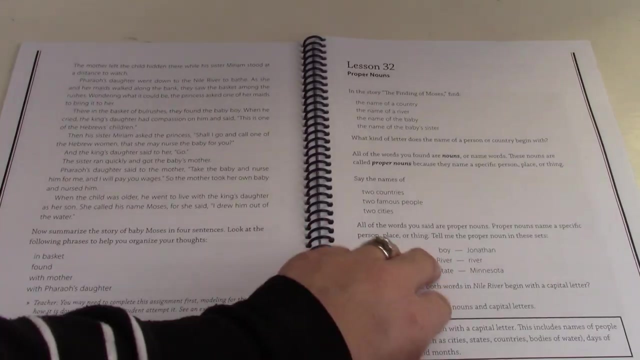 And then more dictionary usage. Okay, Letter and plural nouns: Doing a dialogue- I remember doing that lesson. Oral narration, So a story on the finding of Moses. Proper nouns: Ooh, look at this one, I like this one. 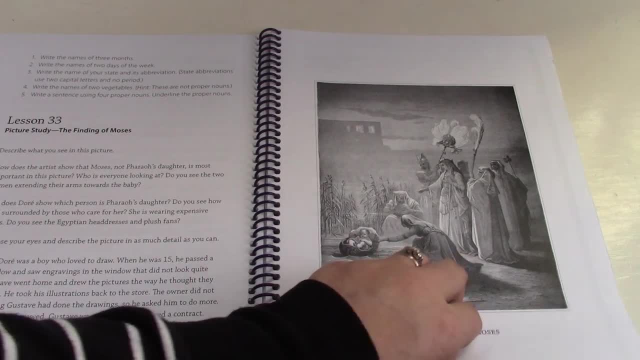 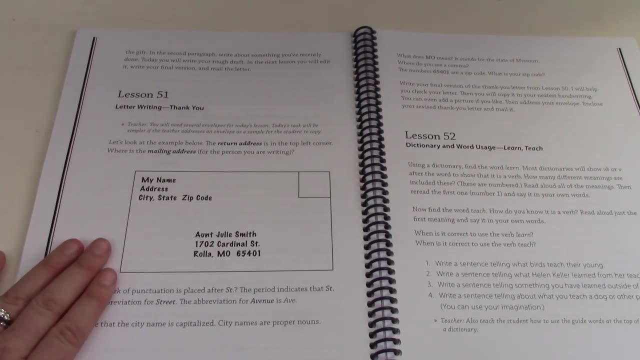 The finding of Moses. Isn't it pretty. I really like that artist. Okay, More oral composition. Let's see More letter writing. Now, this time you know they're actually addressing. you know they're addressing their envelope. 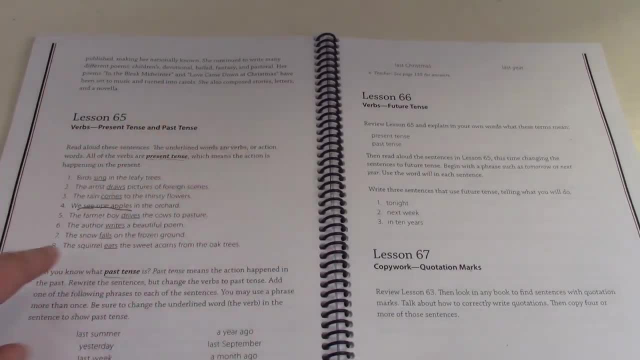 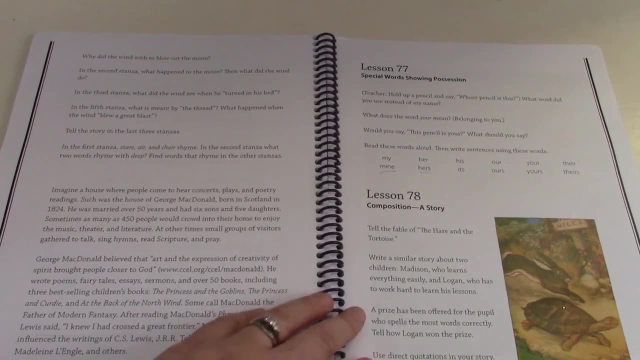 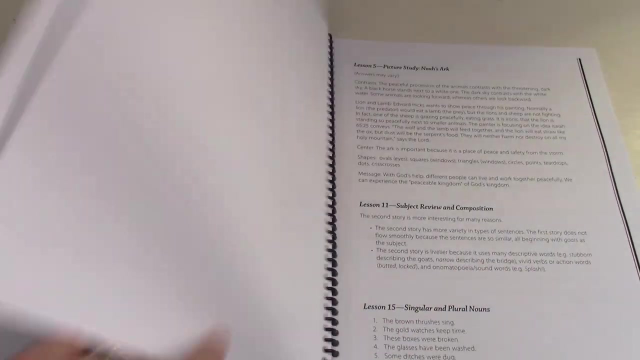 More dictionary usage. Remember, it's just building upon itself. So verbs, We've got present tense, past tense, future tense, More composition mark. There you go, And there's the answers in the back. Okay, so last one that I have. 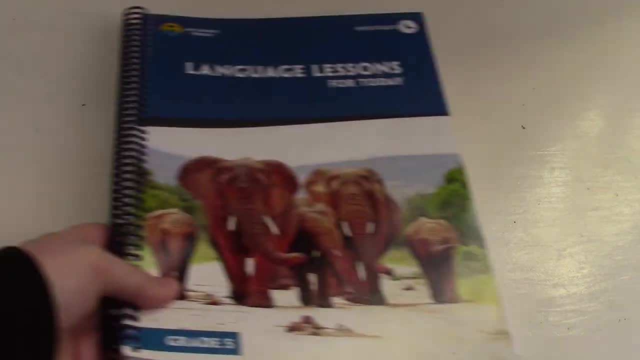 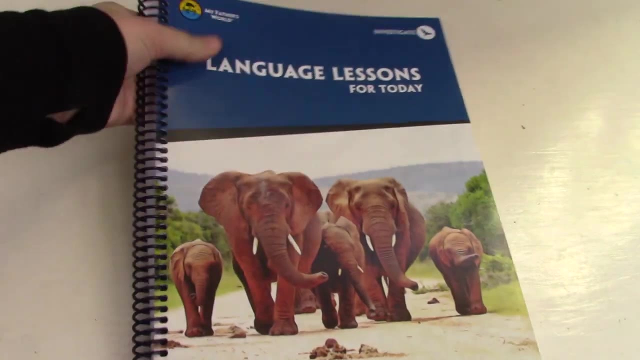 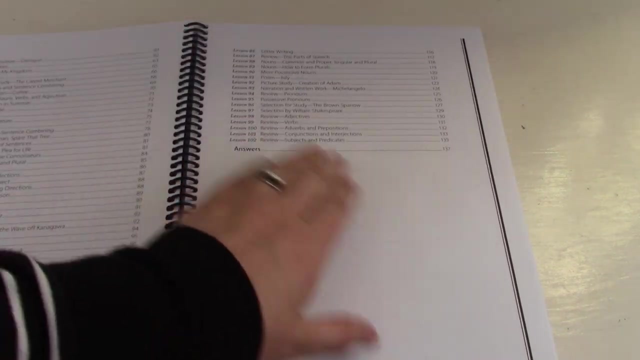 Now remember it goes all the way to grade six. But here is grade five Language lessons for today. Now I definitely notice a difference with the fifth grade. It's definitely thicker. Okay, again, your contents. It goes all the way to 102 lessons. 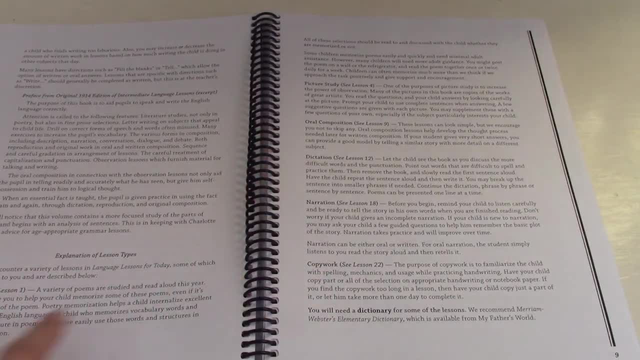 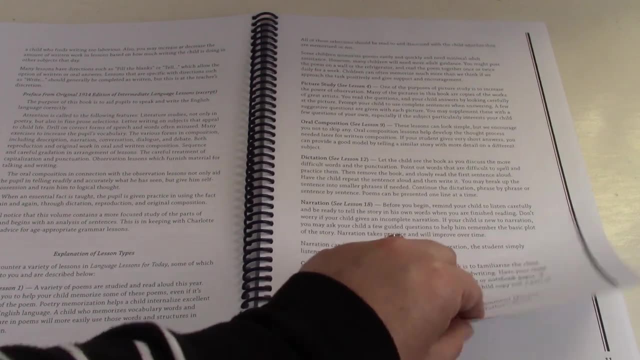 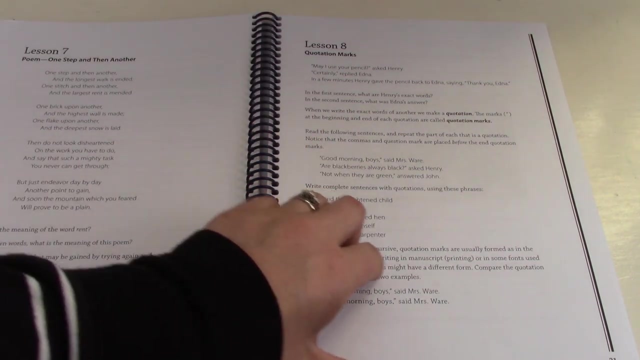 Your introduction And again your explanation of lesson types is the same. This one goes a little bit more to the kind of dictionary you will need And we hop right in back into poems, Quotation marks, Dictation and capitalization. 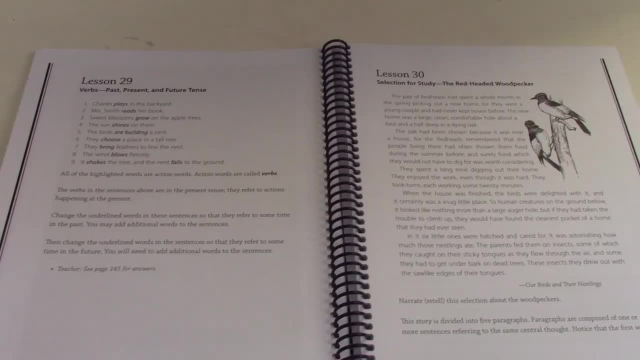 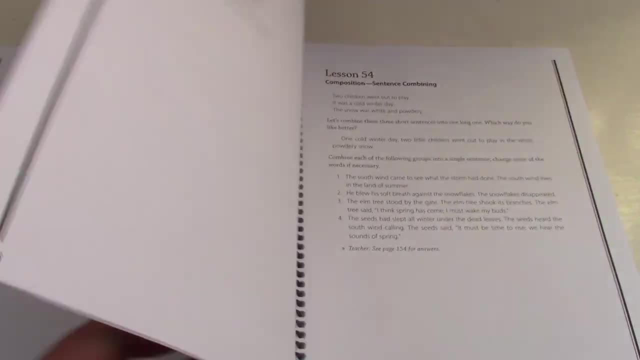 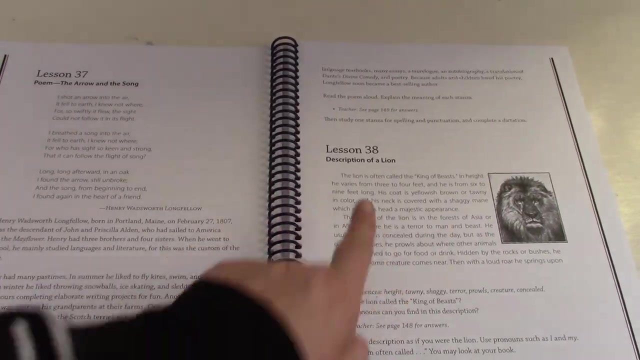 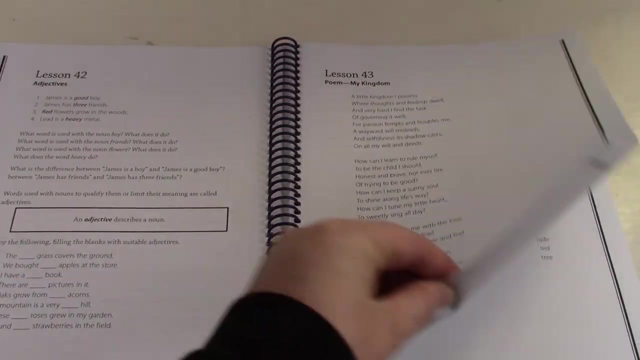 Selections to study abbreviations. Here's more stories to study Verbs: Composition, sentence, combining. Let's see if there's a good Oh, a description of a line in Dialogue Poems: adjectives: Oh, look at that picture study. 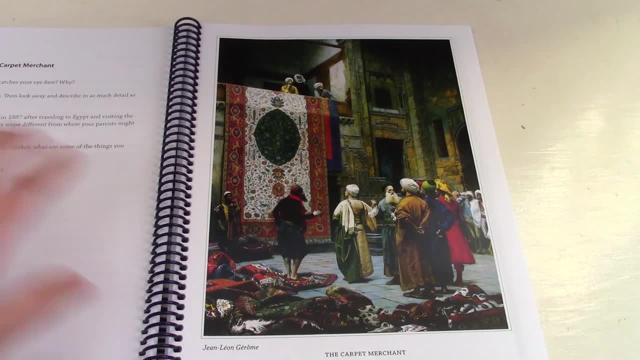 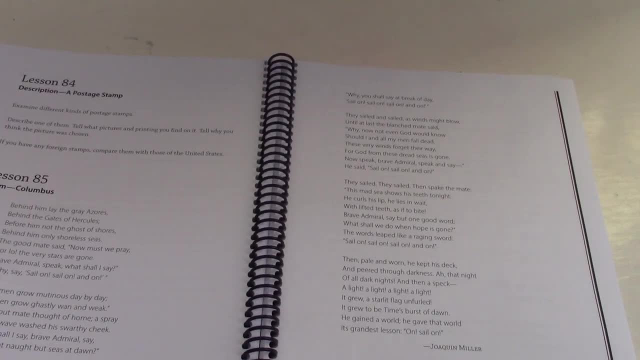 Oh, I'm excited about that one. That's very pretty Okay. verbs a and the. So I've been asked before like: is this enough? Is this really enough? And I really think it is enough. I think it's plenty. 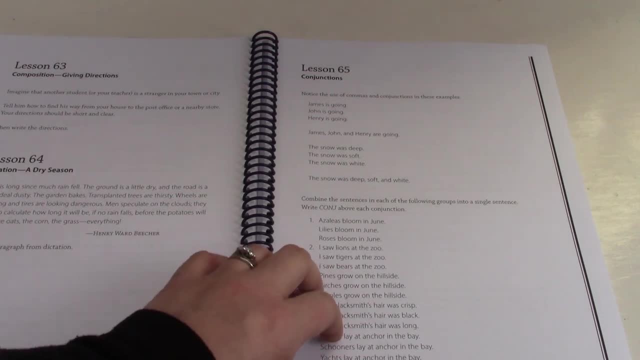 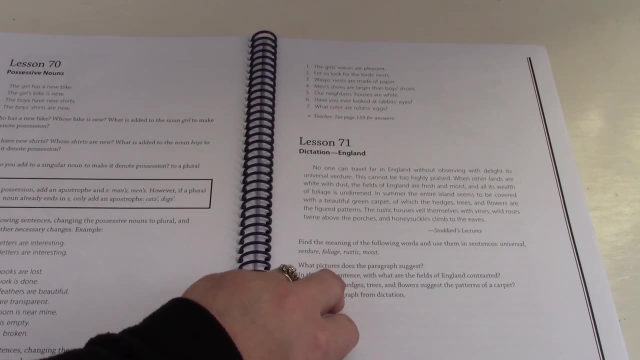 I have found the shorter the lessons, the more they retain. When you're trying to sit with them for so long, they just really start to lose interest and they start to daydream and you just lose them. They're not interested in this, so 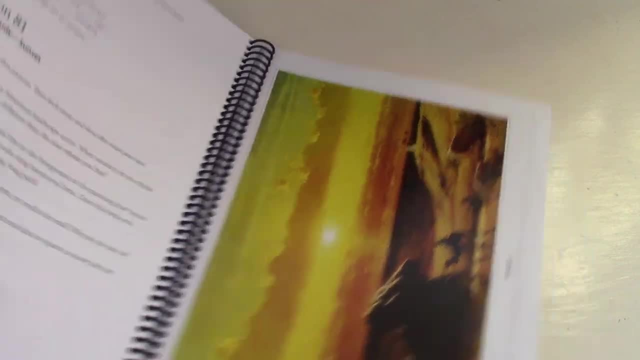 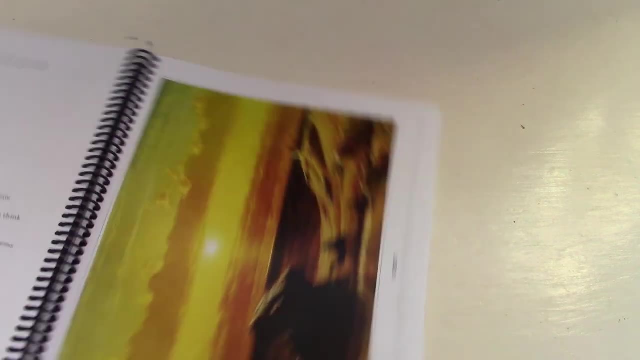 And that's this very Charlotte Mason- to do very short lessons that keep them interested. And then I really think it helps retain more knowledge, which I know does not sound right. Look at that pretty one. Okay, so we're going into possessive prone negative. 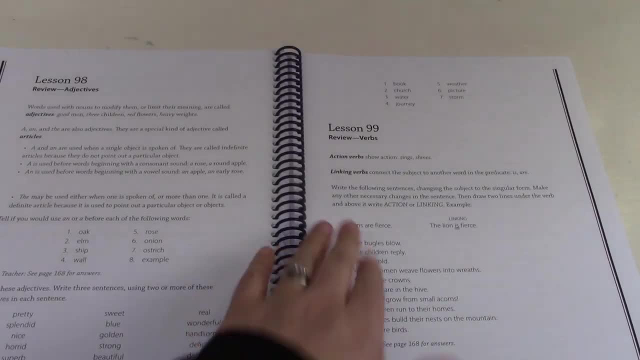 Okay, so we're going into possessive prone negative. Okay, so we're going into possessive prone negative. More studies, verb reviews adjectives. More studies, verb reviews adjectives. Oh, back to the answer keys. 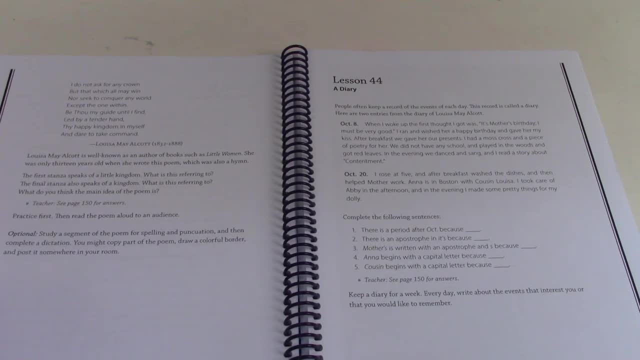 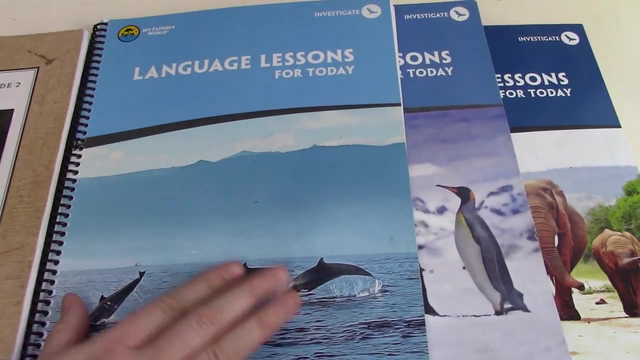 So there you go. That is the fifth one. Ooh, a diary. They can learn how to keep a diary. That will be fun. So again, we just love language lessons for today. I think that it's a great language arts program. 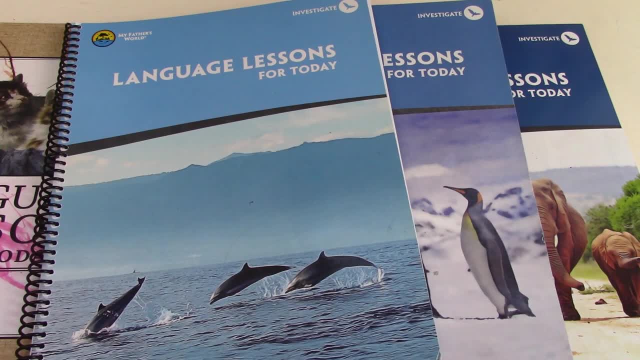 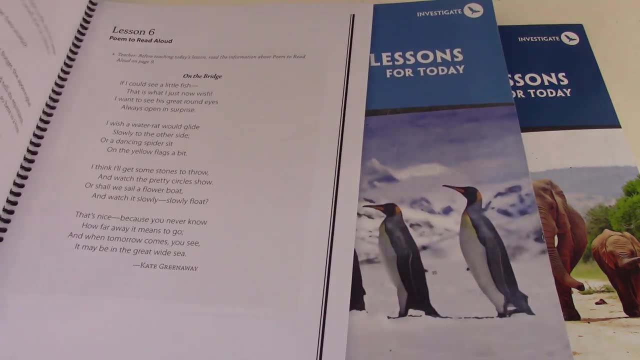 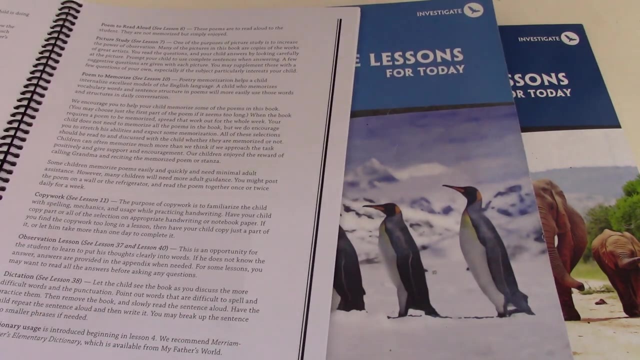 to really help solidify those grammar practices and just learning how to communicate. really that's what language lessons is is communicating in different ways, with writing and doing copy work they have, and observing and dictating, and learning how to look through a dictionary. 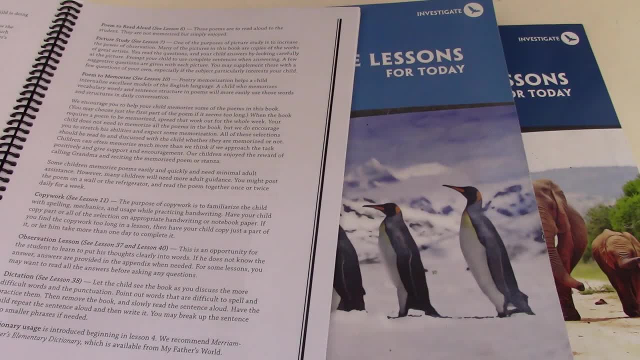 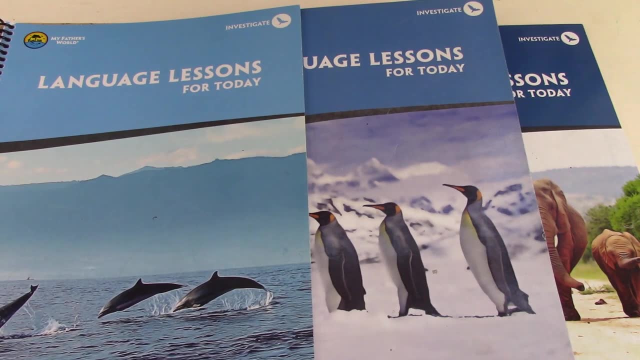 and studying pictures, having a critical eye. I just think it's great, So I hope this video was helpful for you. If you have any questions, please leave them down below, and I hope to see you at the next video. All right, thanks, bye-bye.